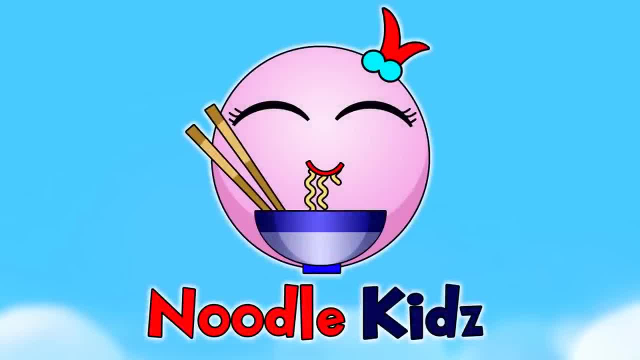 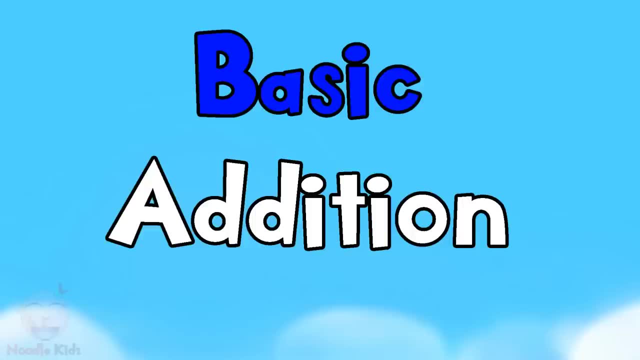 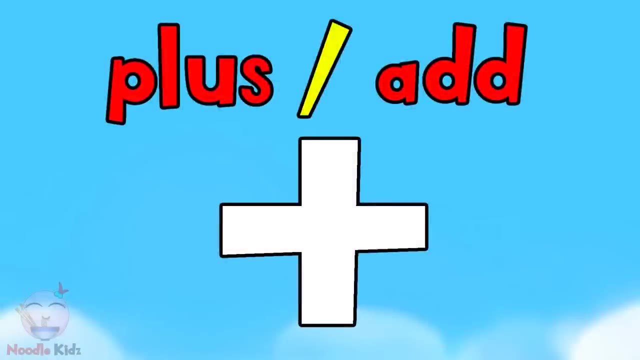 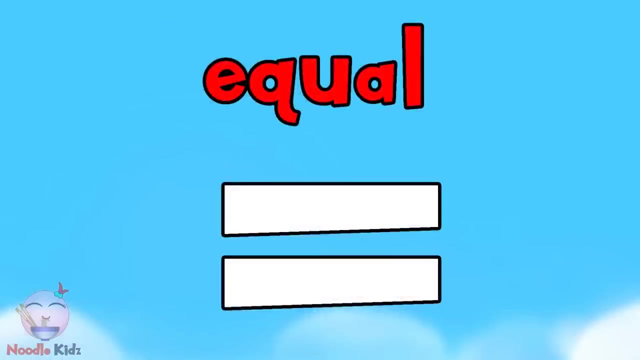 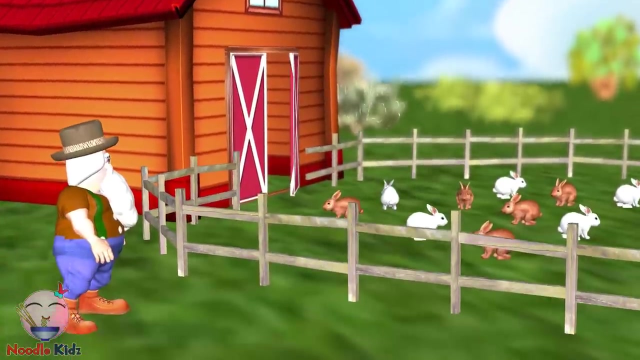 Hi, today we learn about addition. We will do the counting using equation objects and fingers. This is plus. It is used for addition And this is equal. It means it is the result of the counting. Let's go to Uncle Old McDonald's farm and help him count his rabbits. 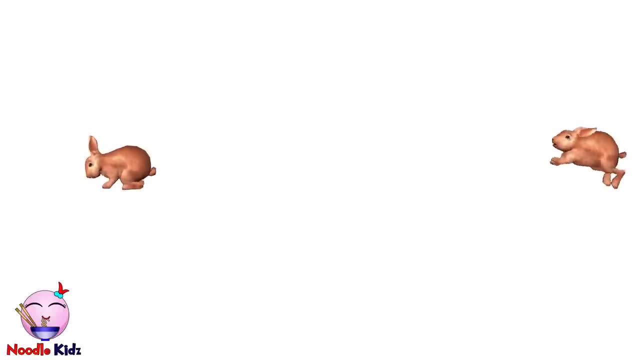 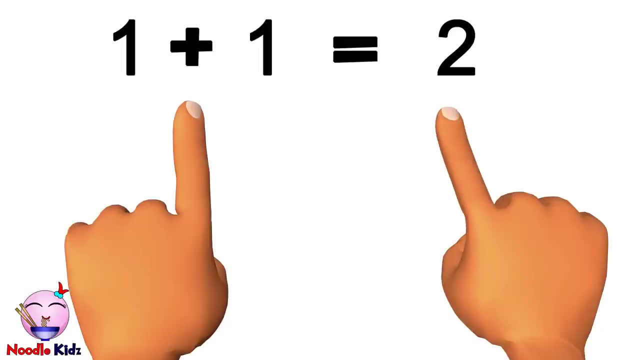 There is one rabbit on the farm, Let's add another rabbit. Let's add another rabbit. Now we have one rabbit plus one rabbit equals two rabbits. In equation, it is one plus one equals two. You can use your fingers too. One finger plus one finger equals two fingers. 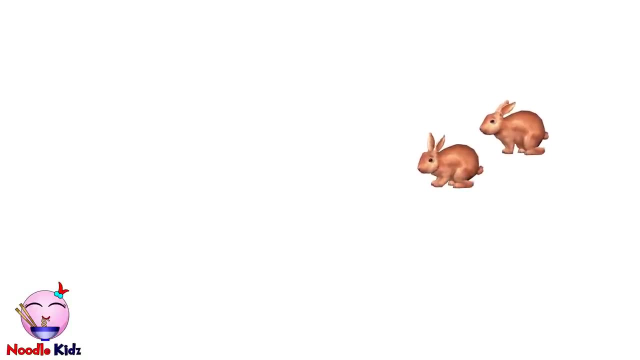 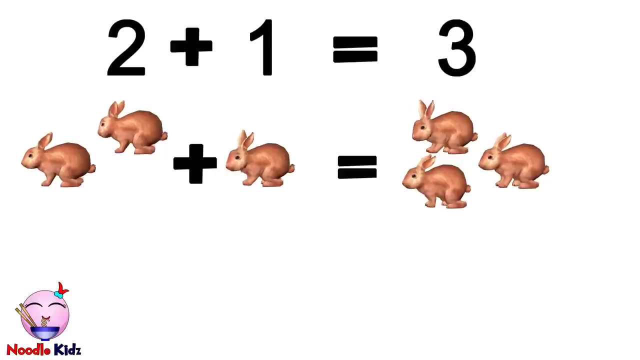 Let's go back to the farm. Now we have two rabbits. Let's add another rabbit. Two rabbits plus one rabbit equals three rabbits. This means two plus one equals three. Let's use our fingers: Two fingers on this hand, One finger on this hand. 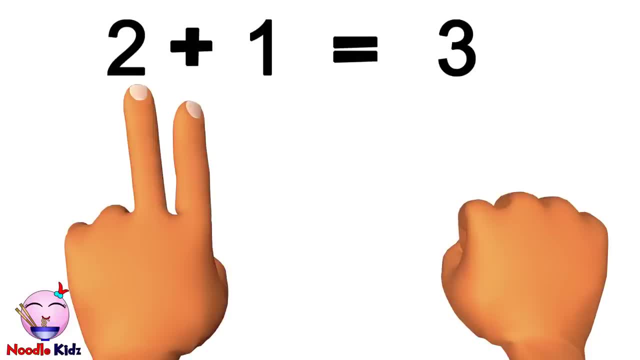 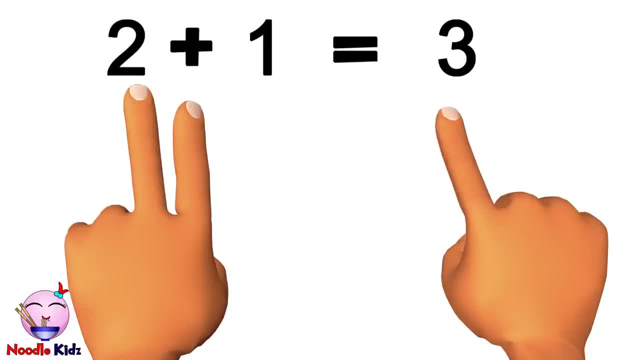 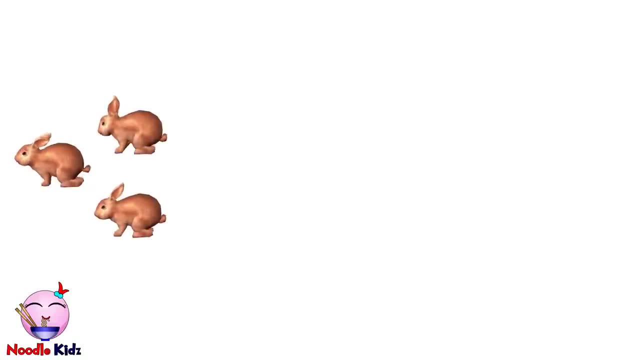 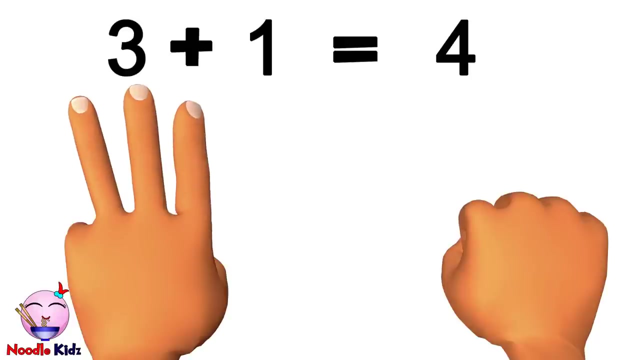 Two fingers on this hand, One finger on this hand. finger on this hand, Two fingers plus one finger equals three fingers. We have three rabbits on the farm. now Let's add another rabbit. Three rabbits plus one rabbit equals four rabbits. It means three plus one equals four. Three fingers plus one finger equals four. 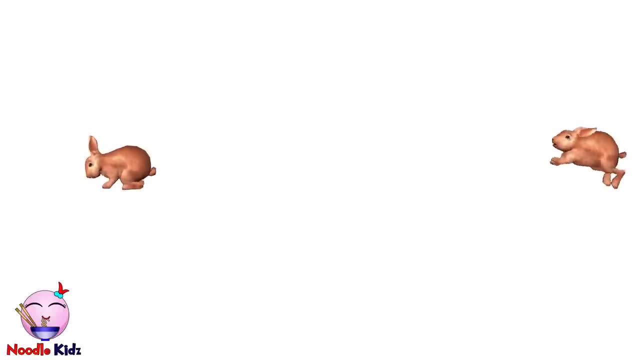 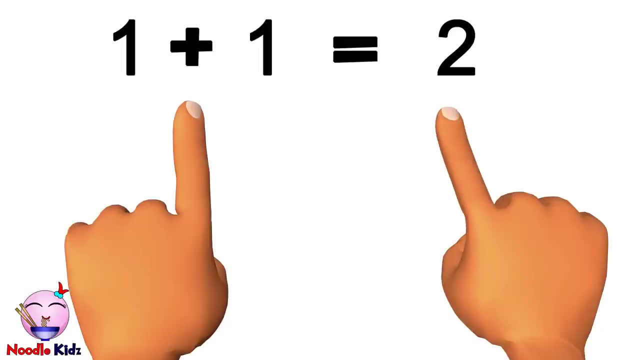 There is one rabbit on the farm, Let's add another rabbit. Let's add another rabbit. Now we have one rabbit plus one rabbit equals two rabbits. In equation, it is one plus one equals two. You can use your fingers too. One finger plus one finger equals two fingers. 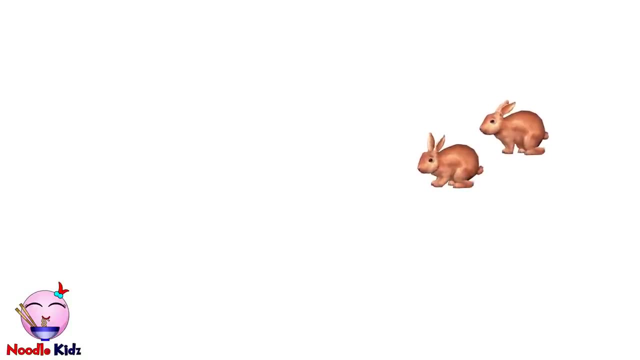 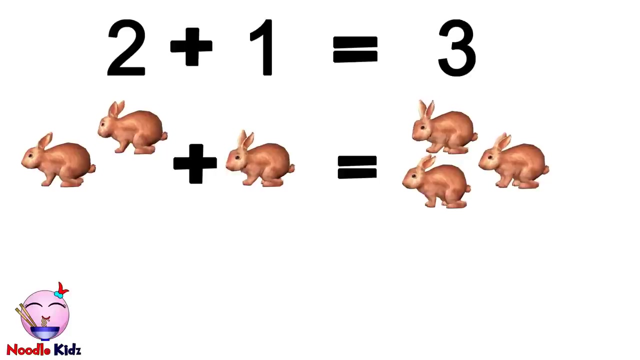 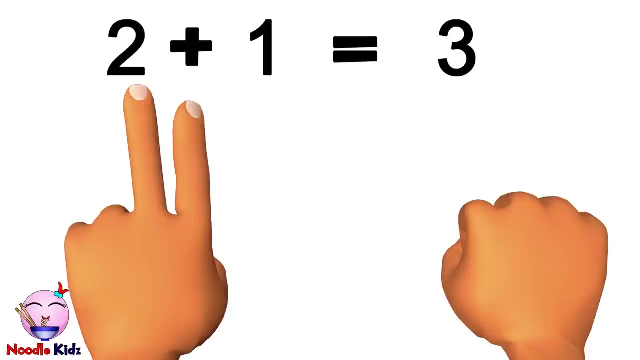 Let's go back to the farm. Now we have two rabbits. Let's add another rabbit. Two rabbits plus one rabbit equals three rabbits. This means two plus one equals three. Let's use our fingers: Two fingers on this hand, One finger on this hand. 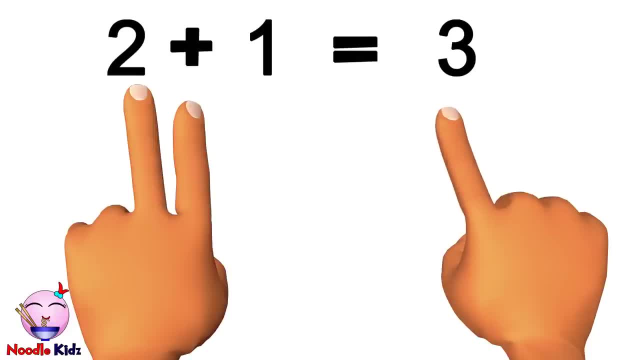 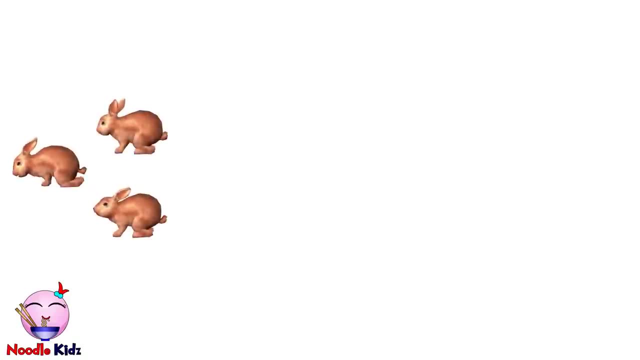 And two fingers on this hand, One finger on this hand. Two fingers plus one finger equals three fingers. We have three rabbits on the farm. now Let's add another rabbit. Three rabbits plus one rabbit equals four rabbits. It means three plus one equals four. 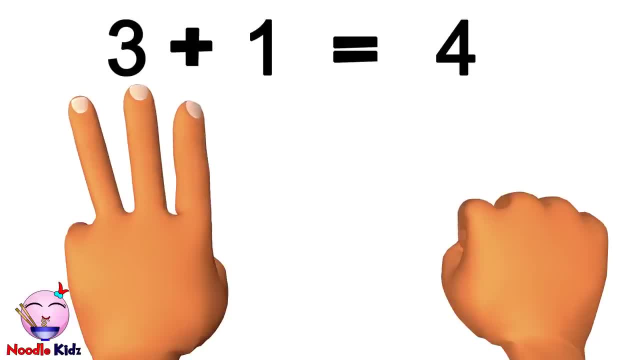 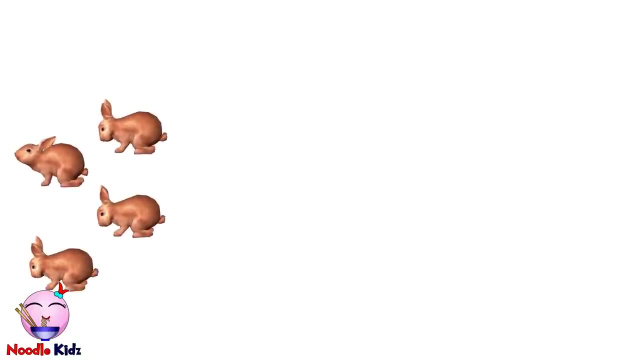 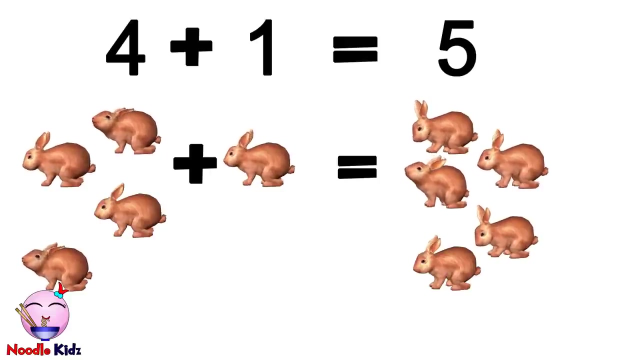 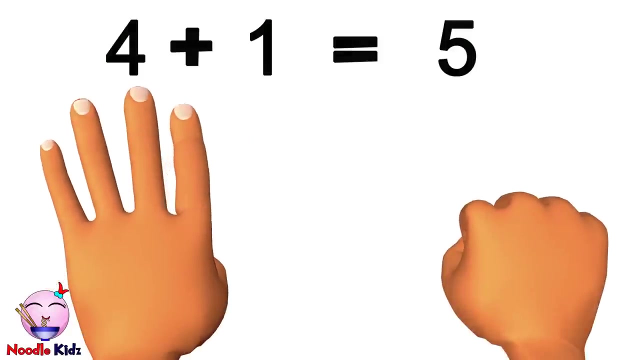 Three fingers plus one finger equals four fingers. Let's go back to the farm. Four rabbits plus one rabbit equals five rabbits. This means four plus one equals five. Four fingers add one finger equals five fingers. This means four plus one equals five fingers. 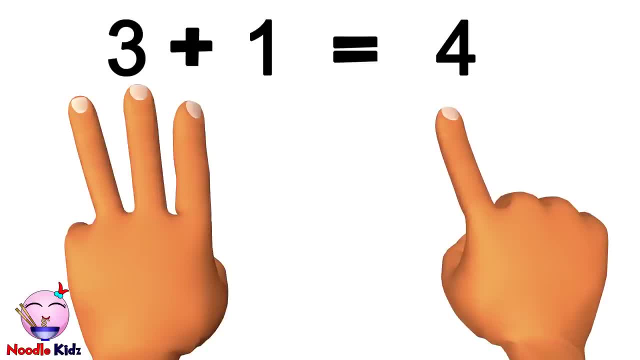 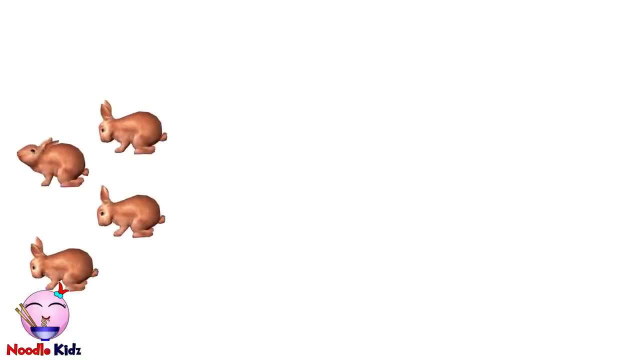 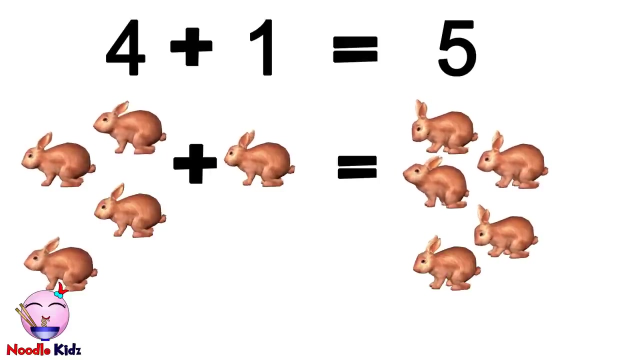 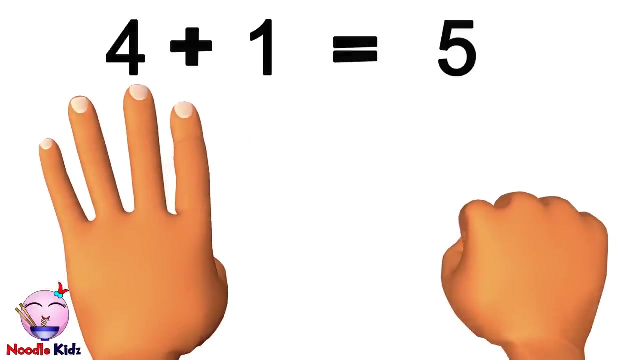 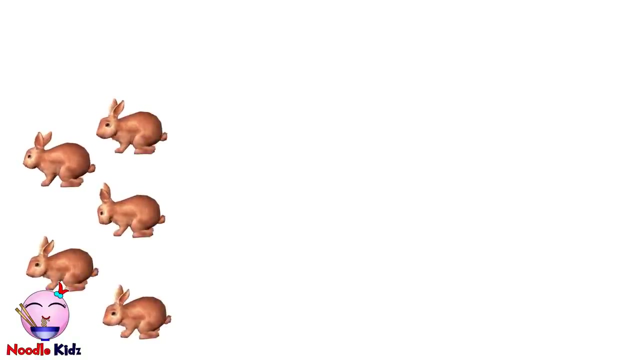 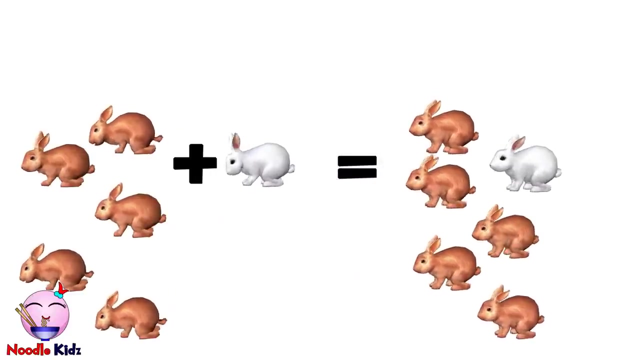 fingers. Let's go back to the farm. Four rabbits plus one rabbit equals five rabbits. This means four plus one equals five. Four fingers: add one finger equals five. Four fingers- add one finger equals five fingers. Five rabbits and one rabbit equals six rabbits. 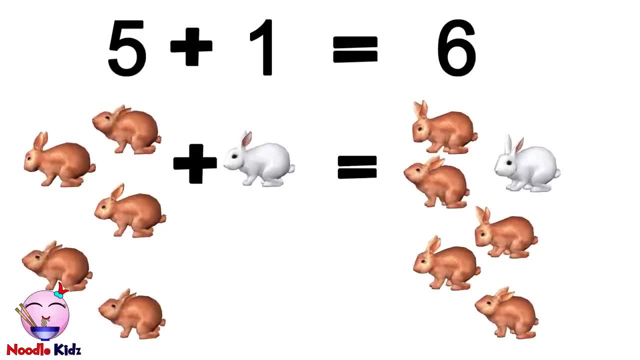 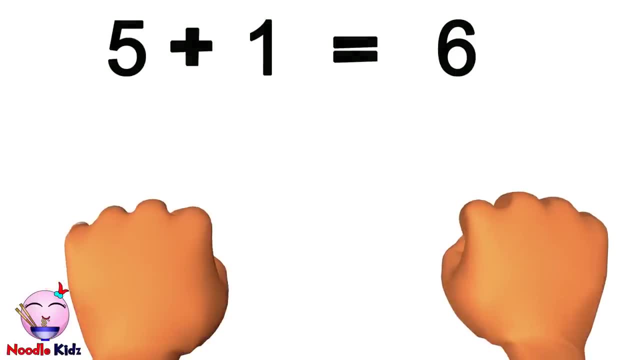 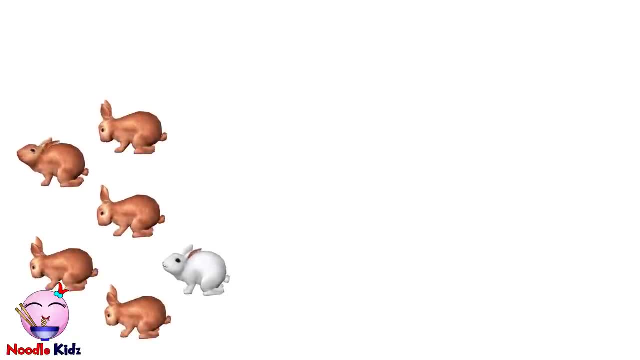 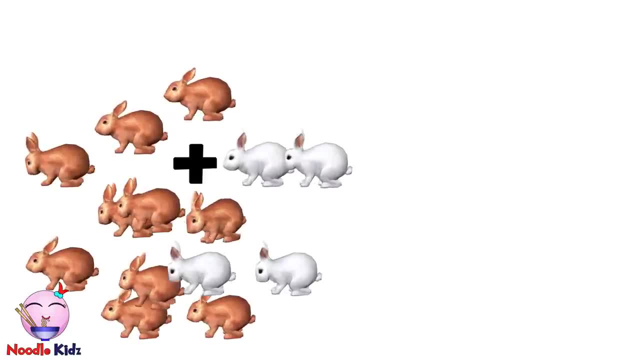 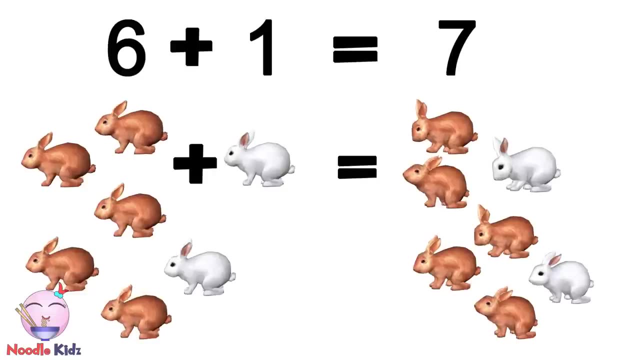 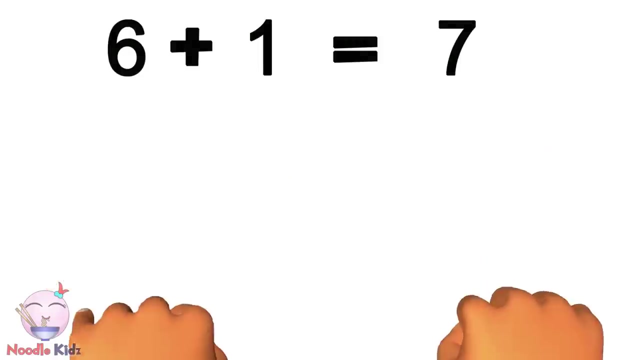 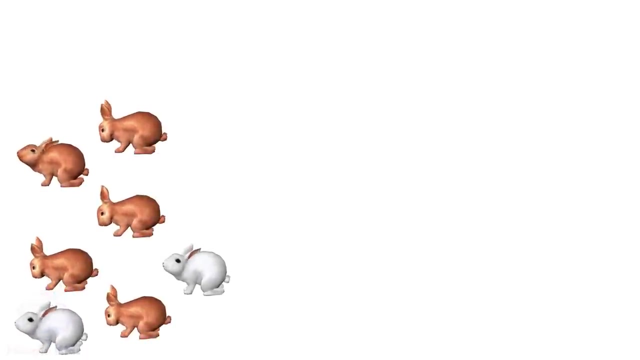 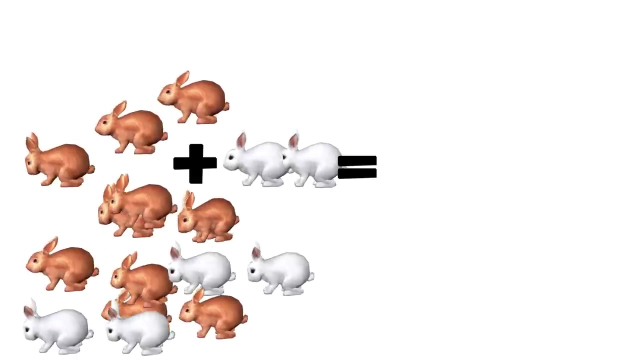 Five fingers add one finger equals six. Five fingers add one finger equals six. Add 1 rabbit equals 7 rabbits, which means 6 plus 1 equals 7.. 6 fingers Add 1 finger equals 7 fingers, 7 rabbits. Add 1 rabbit equals 8 rabbits. 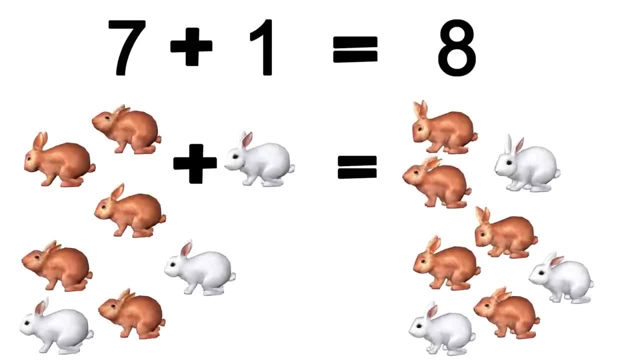 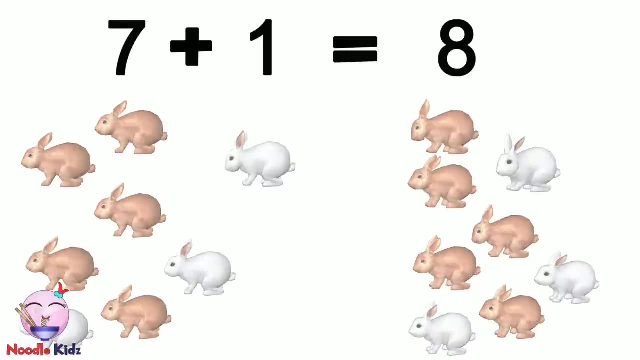 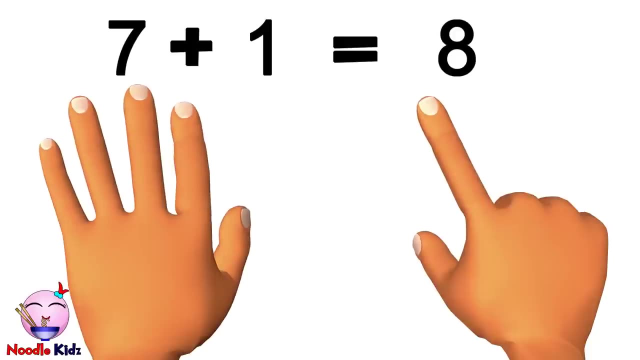 This means 7 plus 1 equals 8.. 7 fingers Add 1 finger equals 8 fingers, 8 rabbits. Add 1 rabbit equals 2 rabbits. 7 fingers Add 1 finger equals 3 rabbits. 1 rabbit equals 3 rabbits. 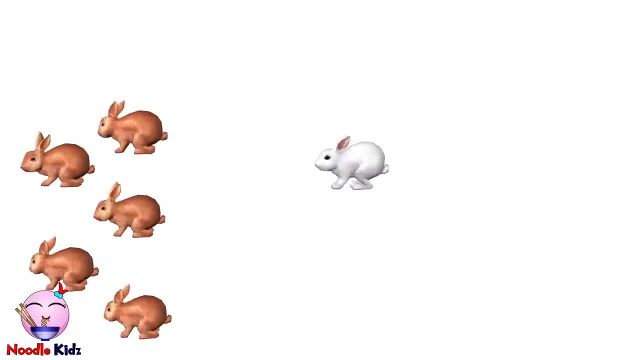 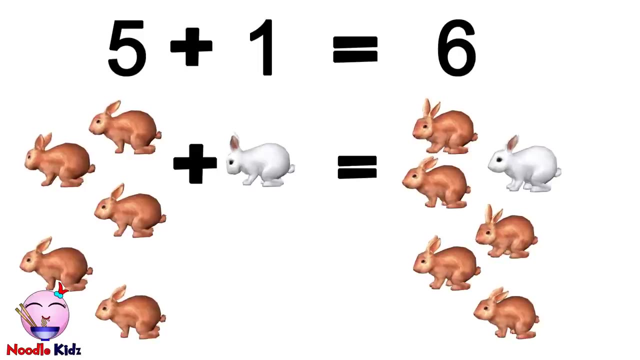 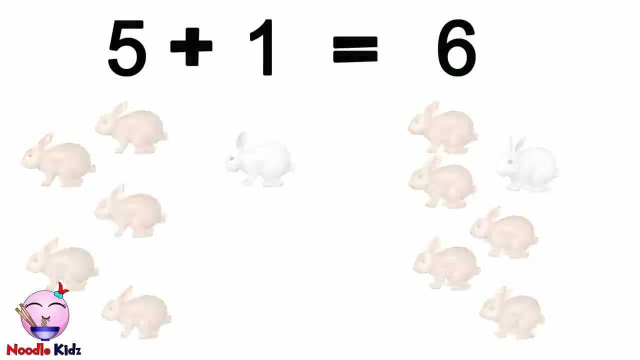 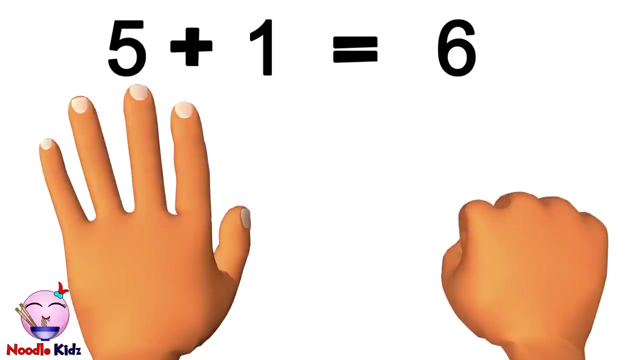 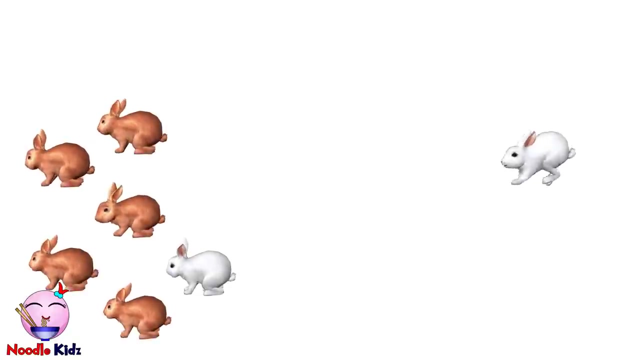 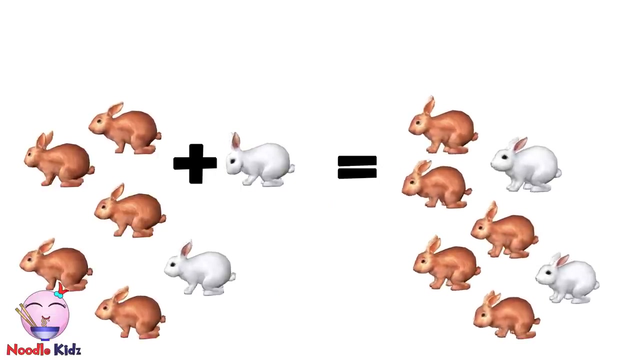 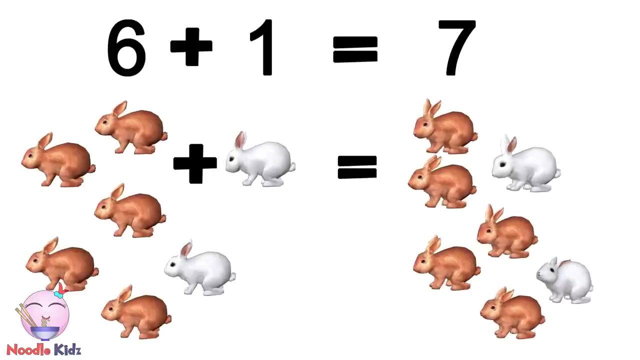 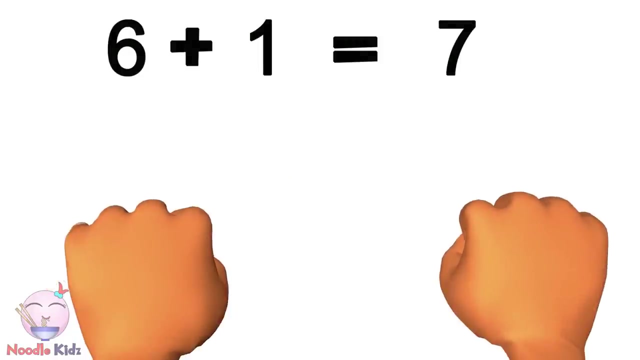 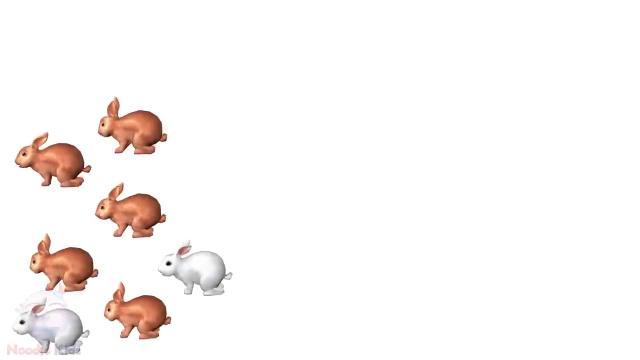 Five rabbits and one rabbit equals six rabbits. This means five plus one equals six. Five fingers add one finger. One finger equals six fingers. Six rabbits. Add one rabbit equals seven rabbits, Which means six plus one equals seven. Six fingers Add: one finger Equals seven fingers. 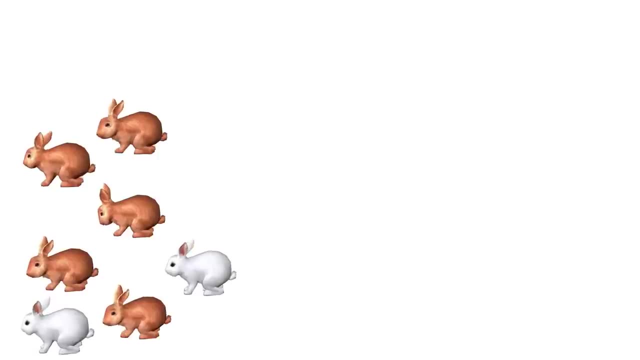 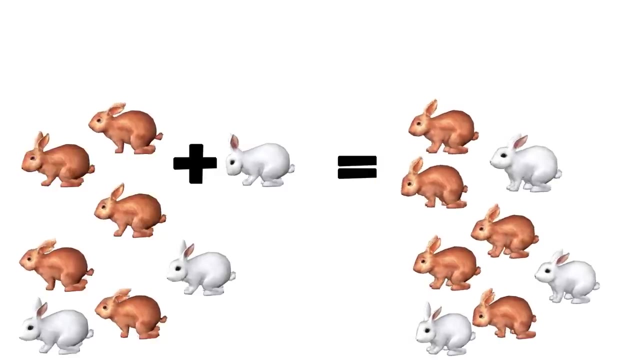 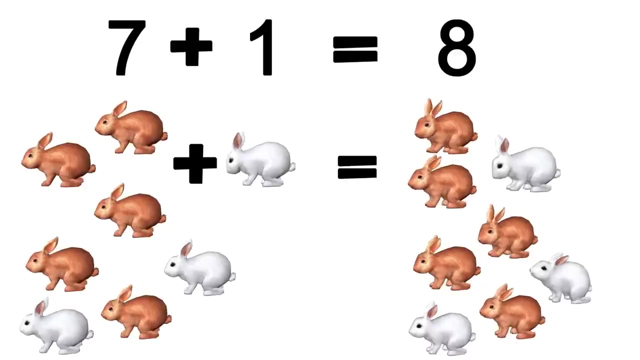 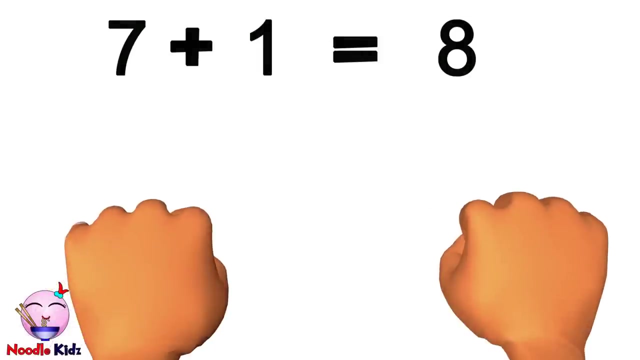 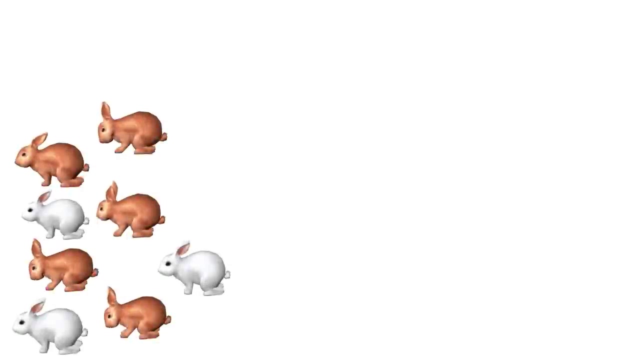 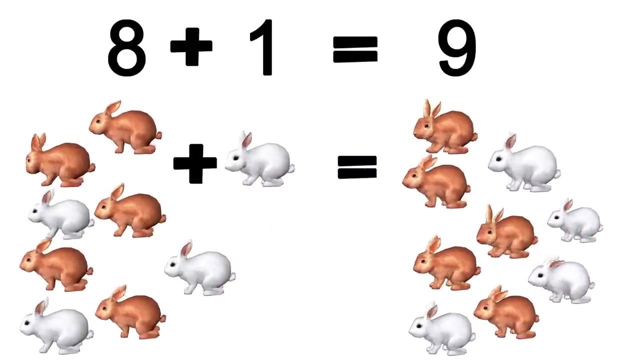 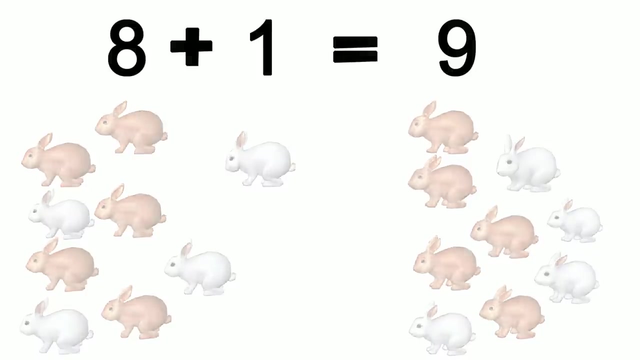 Seven rabbits Add one rabbit Equals eight rabbits. This means seven plus one equals eight. Seven fingers Add one finger Equals eight fingers. Eight rabbits Add one rabbit Equals nine rabbits. This means eight plus one equals nine. Seven rabbits Add one rabbit Equals eight rabbits. 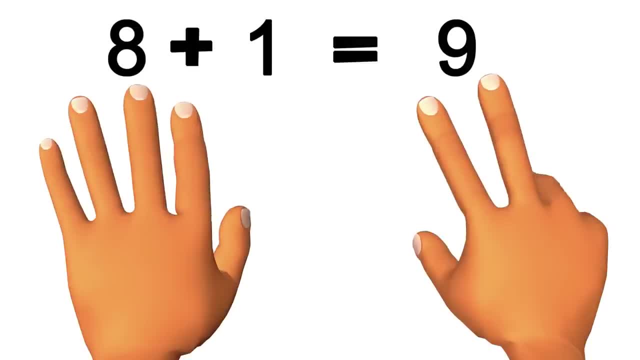 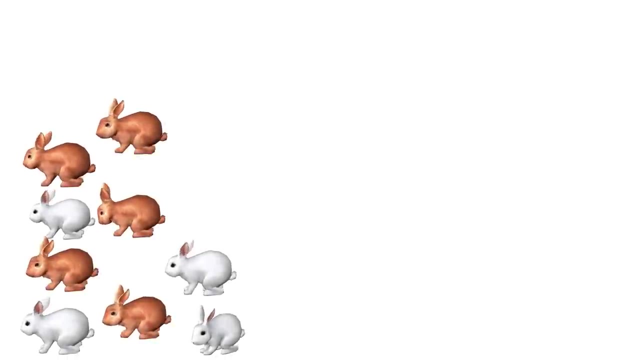 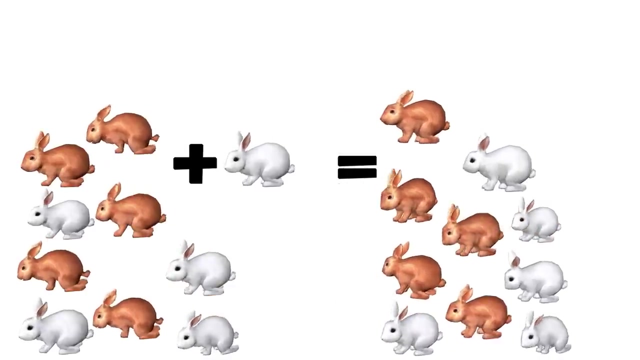 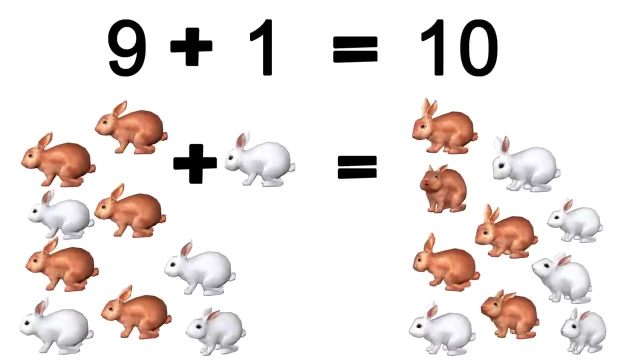 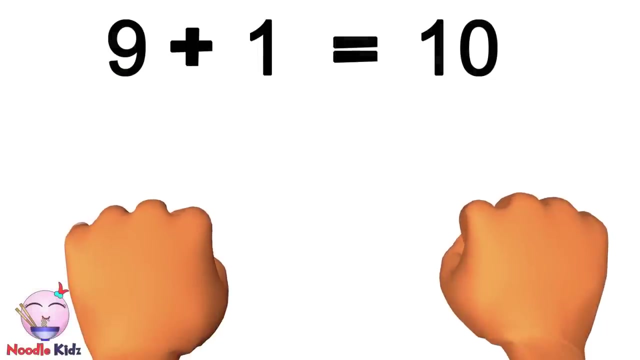 Eight fingers Add one finger Equals nine fingers. Nine rabbits Add one rabbit Equals ten rabbits. This means in equation we have nine plus one equals ten. Nine fingers Add one finger Equals ten fingers. Nine fingers Add one finger Equals ten fingers.